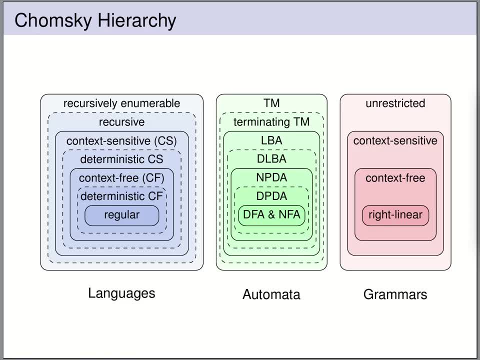 Hierarchy. This is the Chomsky Hierarchy. We have different classes of languages. They correspond to different types of automata and they can be defined via different variants of grammars. The smallest class of languages that we've discussed are the regular languages. 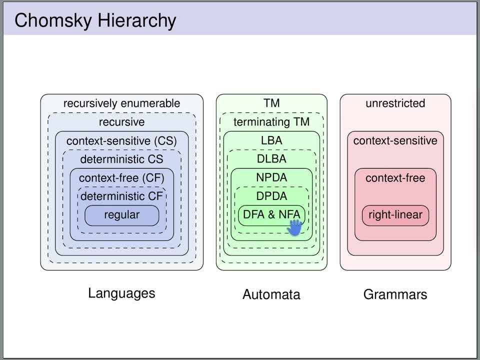 They can be defined via deterministic finite automata and non-deterministic finite automata. Both versions of automata are equally expressive. Their regular languages can also be defined via regular grammars, in particular via Ratelinear grammars. We've seen one more way of defining regular languages in this course, which is not mentioned. 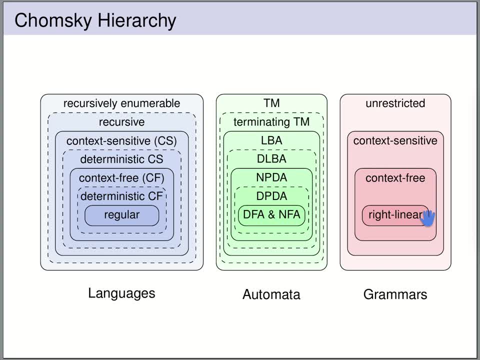 in this slide, and that's the well-known regular expressions. The next bigger classes of languages are the deterministic, context-free and the context-free languages. Let's look at this example 7.1.. weiterrare the言ہ, mitTERR clairement CO. Vietnamese, English, English groups. Augen' lI字ie. 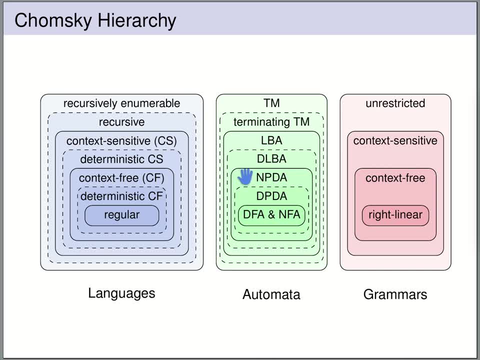 languages can be defined via non-deterministic pushdown automata and equivalently expressive via context-free grammars. There's a subclass of the context-free languages that's strictly in between the regular languages and the context-free ones, that's the deterministic context-free languages. 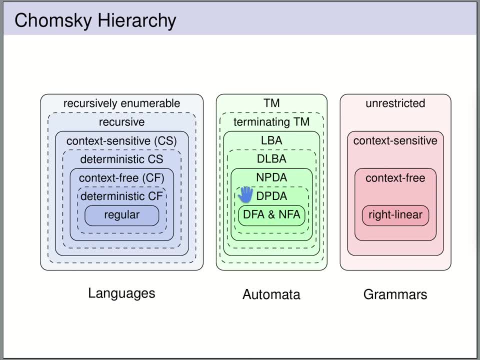 They can be defined via deterministic pushdown automata. The next bigger classes are deterministic, context-sensitive and the context-sensitive languages. The context-sensitive languages can be defined via linear bounded automata. So recall that this is non-deterministic. Turing machines that are not allowed to leave the 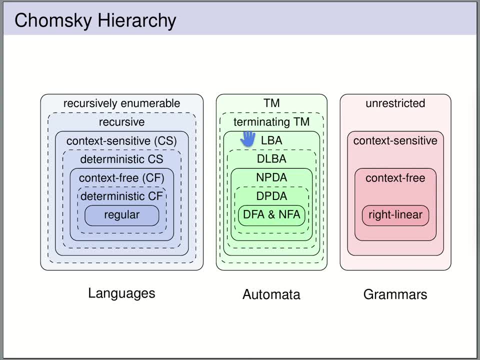 bounds of the input word And equivalently expressive. So let's take a look at the non-deterministic Turing machines, The non-deterministic context-sensitive grammars. these are grammars where the right hand side cannot be shorter than the left hand side. 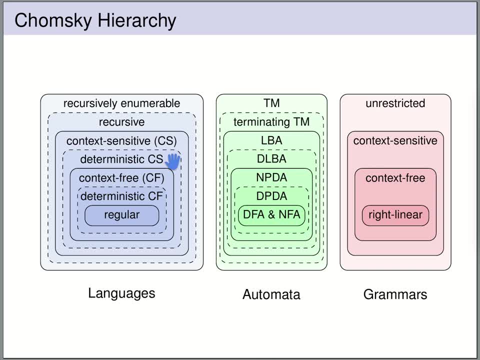 We have, as a subclass of the context-sensitive languages, the deterministic context-sensitive languages, which are defined via deterministic linear bounded automata And actually it's not known whether this is a strict subclass, So it's not known whether the deterministic context-sensitive languages are more expressive.